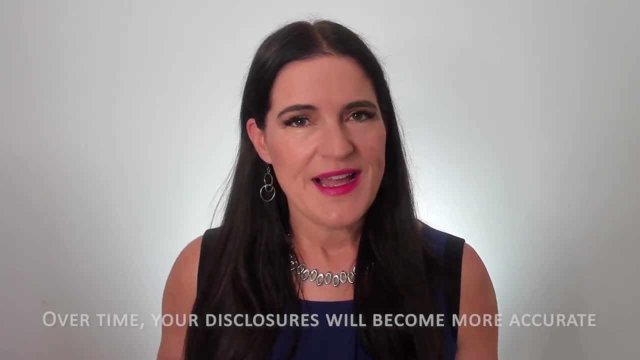 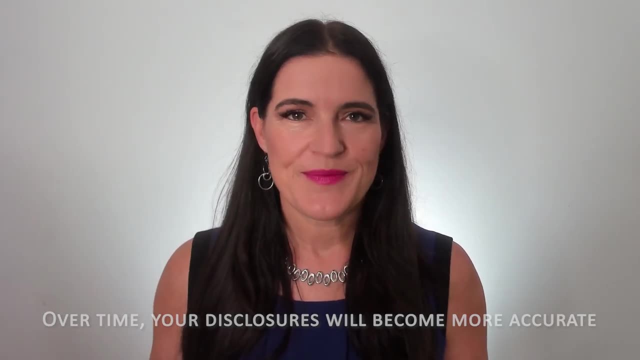 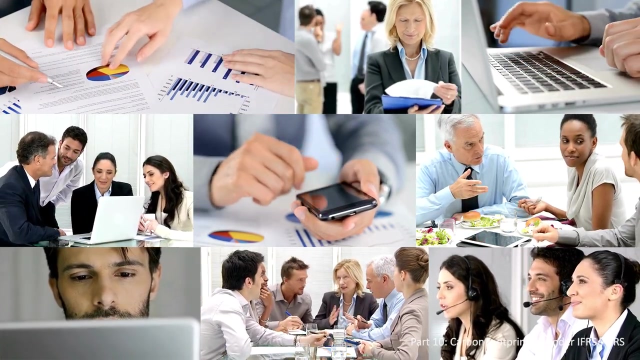 detailed information across the value chain. However, over time, as you enhance your internal capabilities and methodologies, these disclosures are expected to become more accurate. What we have noticed is that some large emitting organisations are starting to collaborate more closely with the value chain to obtain carbon footprint information directly from. 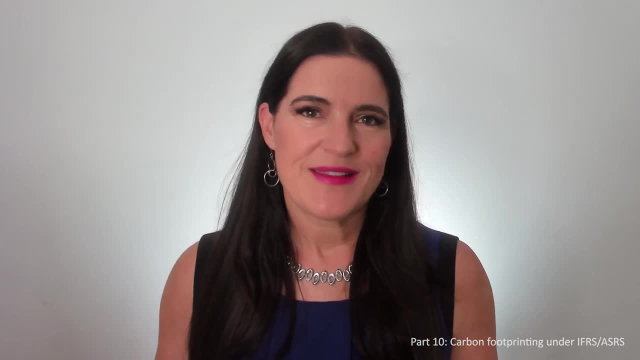 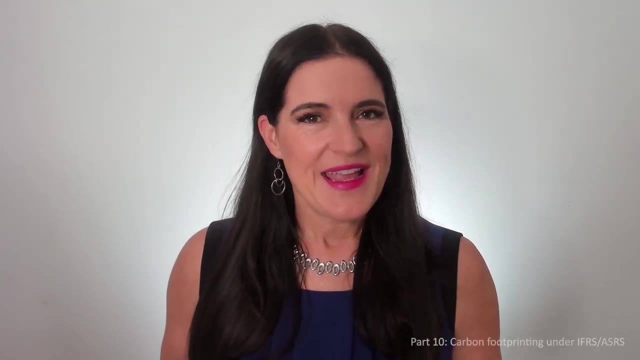 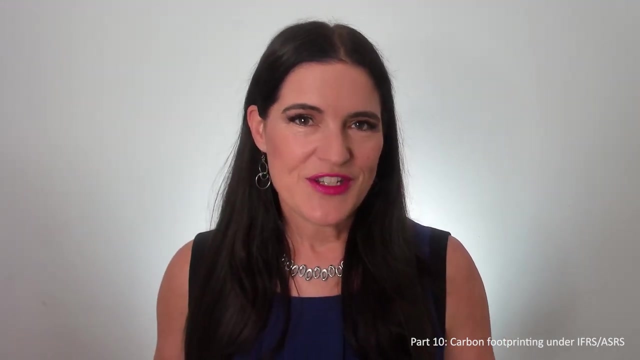 their suppliers. If you are interested in learning more about this collaborative approach, please watch video 8 in this series. The link is in the description. Here are some key considerations for Scope 3 emissions. First up, the good news: You have an additional year to report Scope 3 emissions, acknowledging 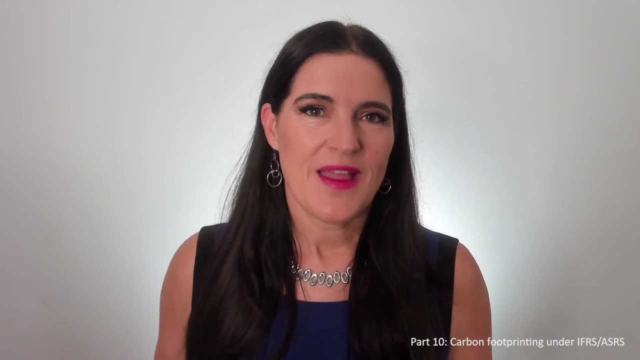 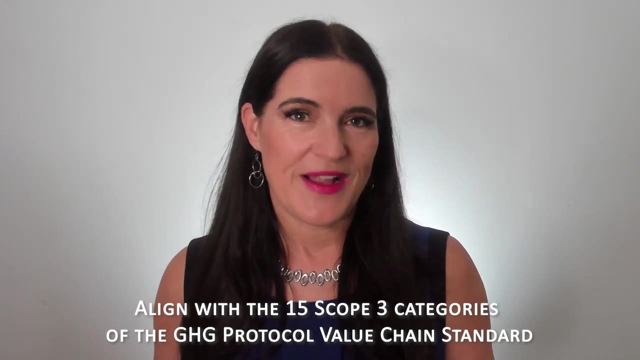 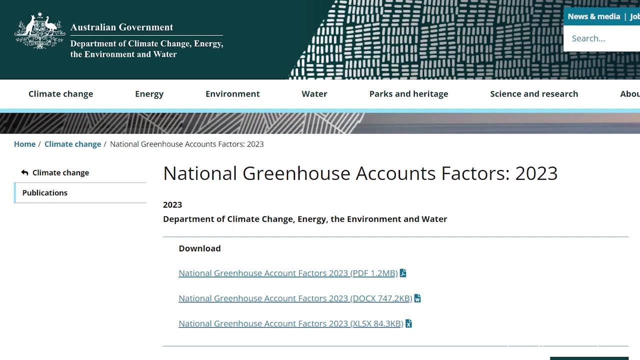 the complexity of these calculations. When you calculate your Scope 3 emissions, you need to align with the 15 categories of the Greenhouse Gas Protocol value chain standard. 1.. In terms of emissions factors, you need to use the national greenhouse accounts factors. 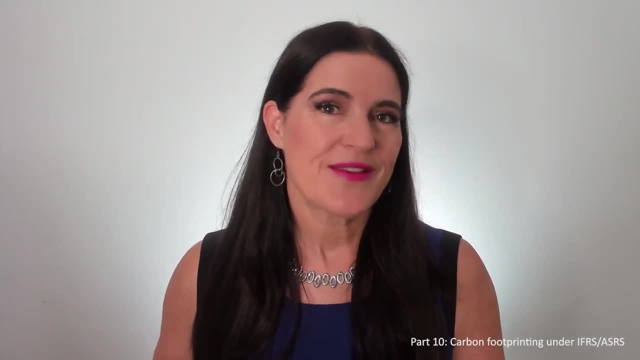 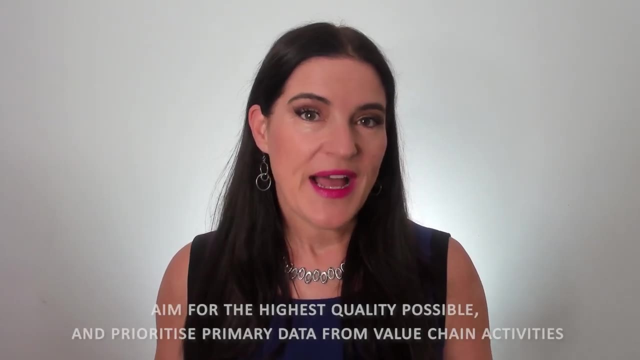 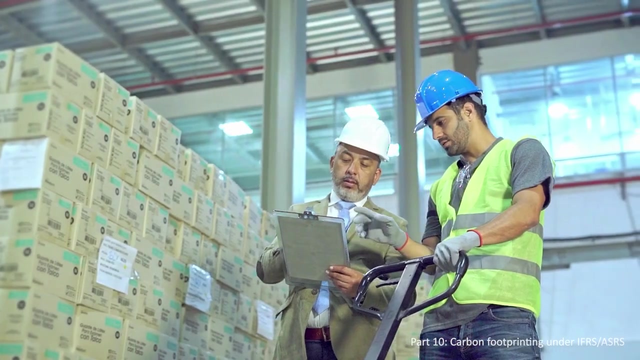 whenever this is possible. Where you can't, you can draw on other Australian sources before applying international factors. In terms of data quality, aim for the highest quality possible and prioritise primary data from value chain activities. Primary data is data obtained directly from specific activities. 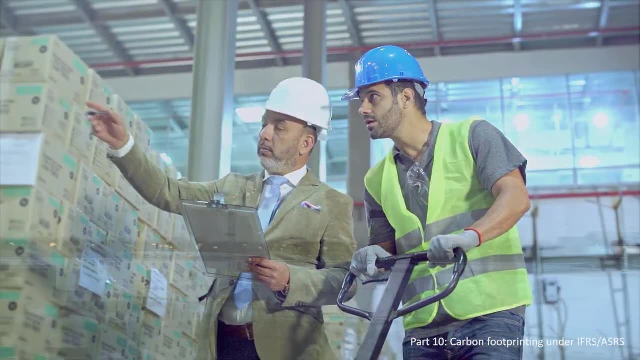 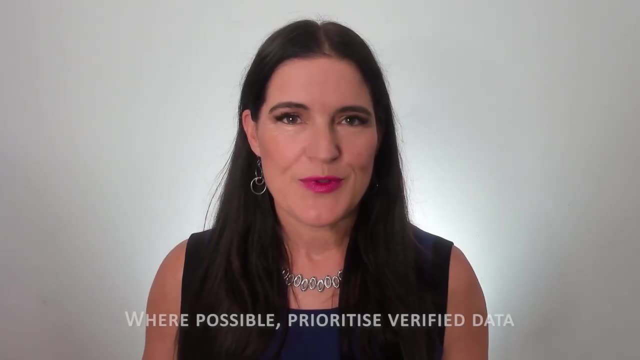 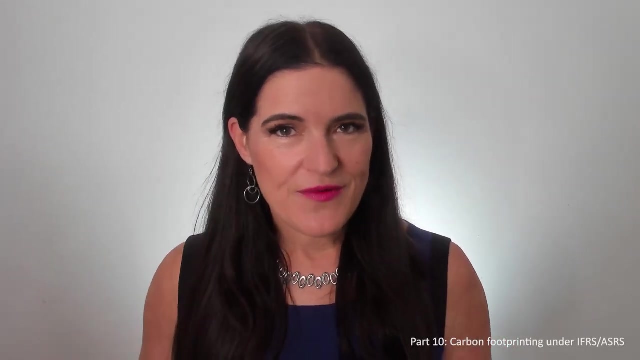 within your value chain, such as supplier-specific emissions factors for purchased goods and services or distance travelled and travel class used by employees when travelling. Where possible, prioritise verified data to enhance the credibility of your reporting. Note that data can be internally verified, such as by reviewing calculations, or externally. 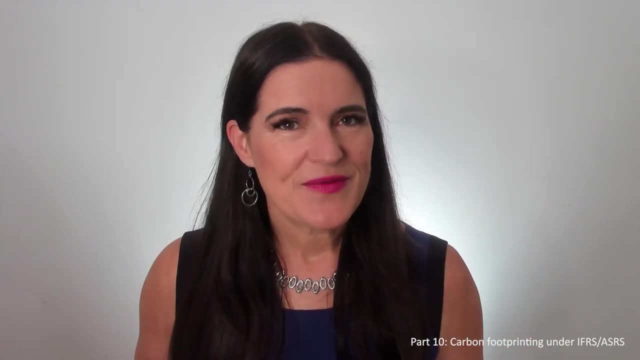 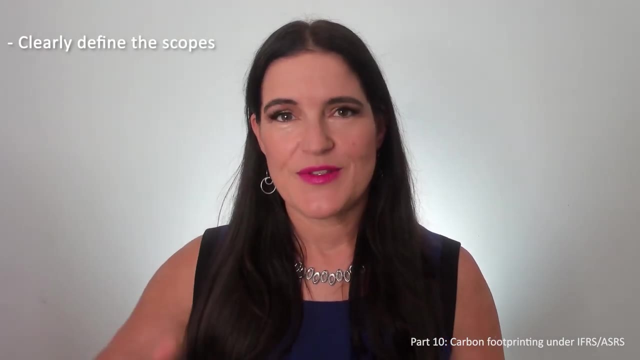 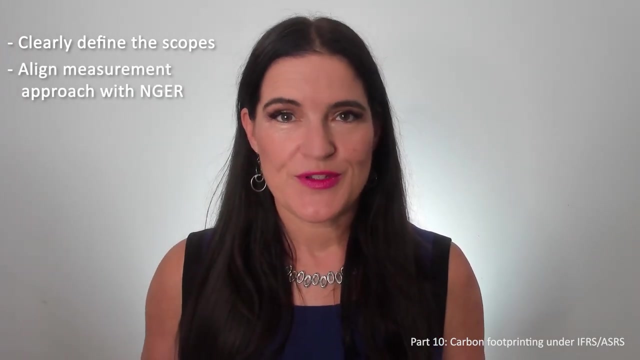 verified via assurance providers. So how can you develop an ESRS compliant carbon footprint? Begin by clearly defining the scope of your emissions, categorising them into Scope 1, Scope 2 and Scope 3.. Align your measurement approach with the ENGA legislation for Scopes 1 and 2.. 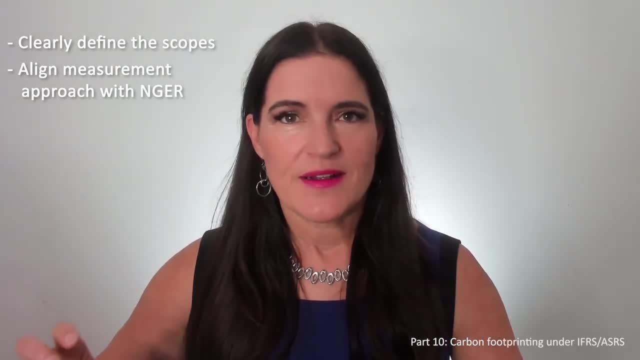 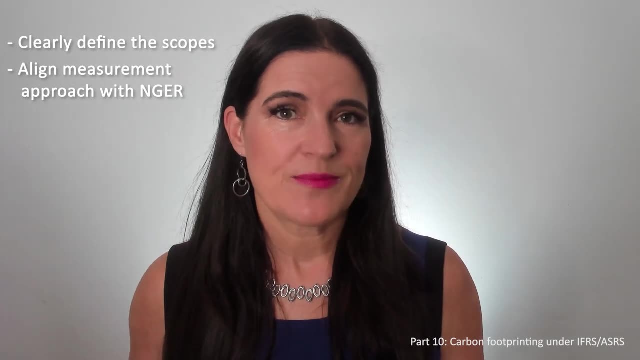 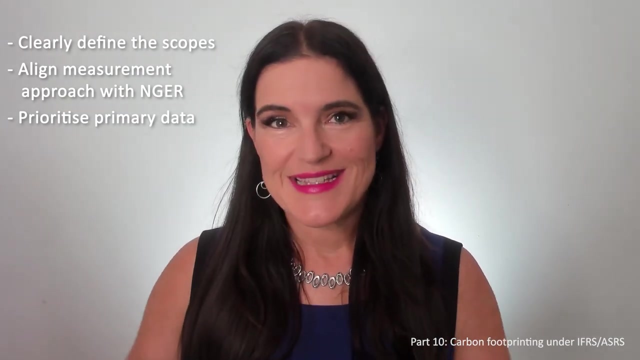 To estimate Scope 3 greenhouse gas emissions, you can use ENGA, for instance, to calculate emissions from your contractor's fuel consumption, and other methods from the Greenhouse Gas Protocol. Collect data across all relevant categories, understanding that, while primary data is ideal,